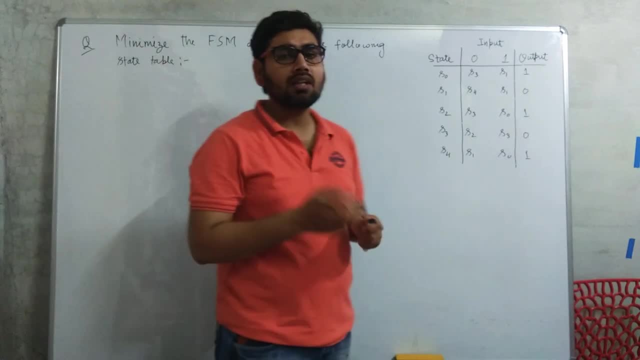 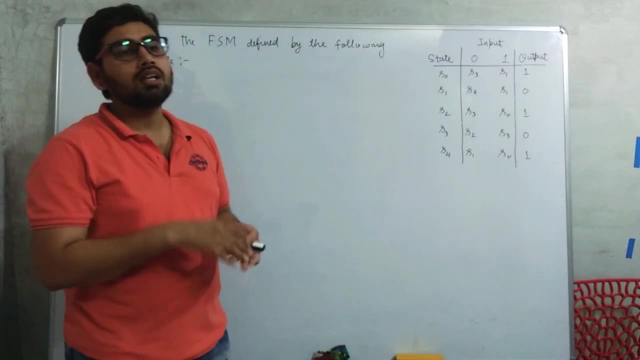 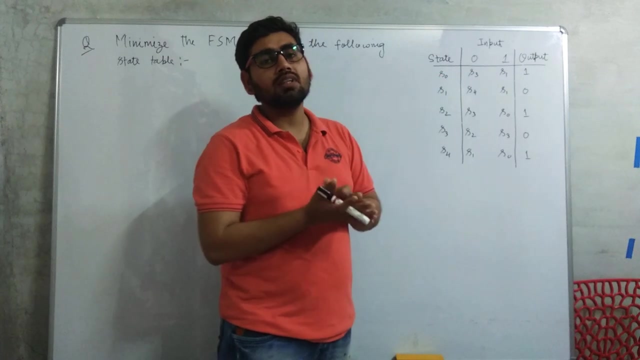 minimization of machines, that in a machine like this, the number of states to be reduced will be its minimized form. How will the number of states be reduced? We have defined the equialent of states. We have said that states are of zero equivalent and we have defined 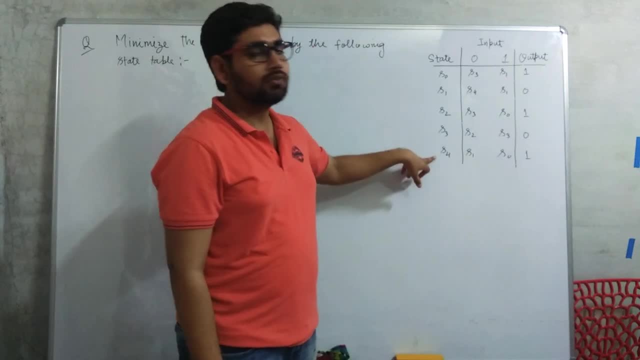 the equalence. From the help of this equal欸, we will reduce the number of states and bring We have 5 states: S0, S1, S2,, S3 and S4. Two inputs: 0 and 1 Output: 1, 0, 1, 0, 1. 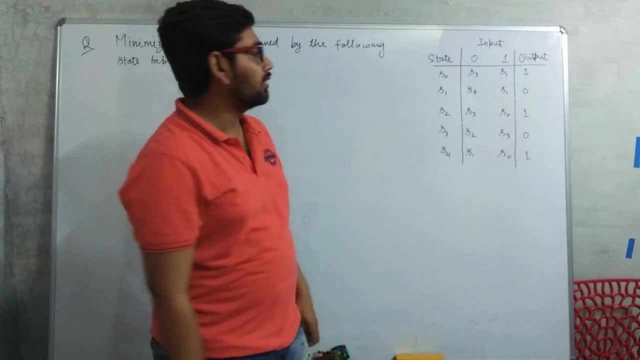 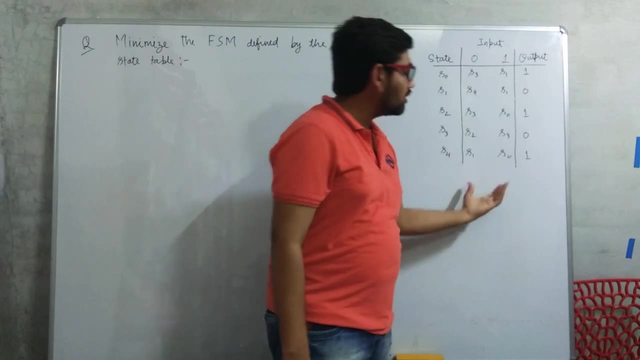 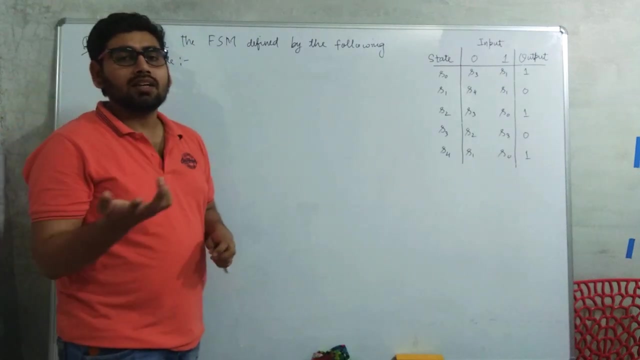 We have different output for each of these states. These transitions are given: S0 gets S3 after giving 0 input. S1 gets S0 after giving 1 input. This way we have given these transitions. We have to bring this in minimized form. To bring this in minimized form, we will define equivalence. 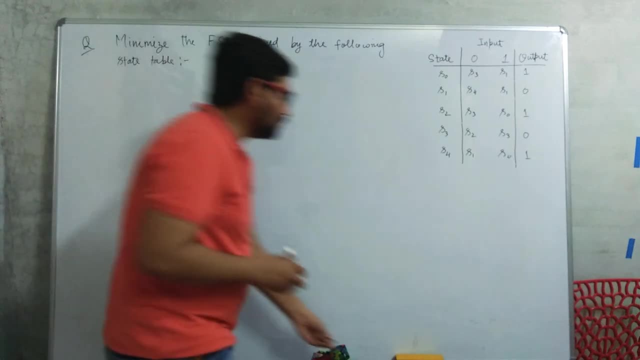 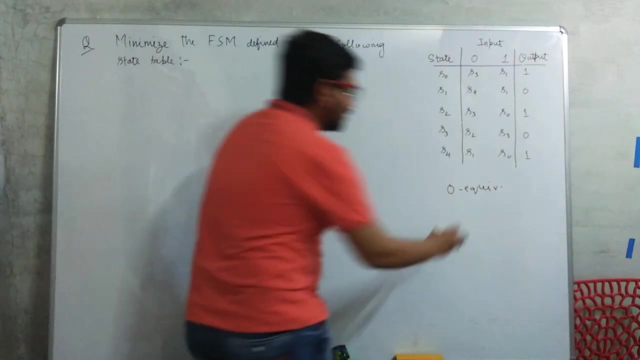 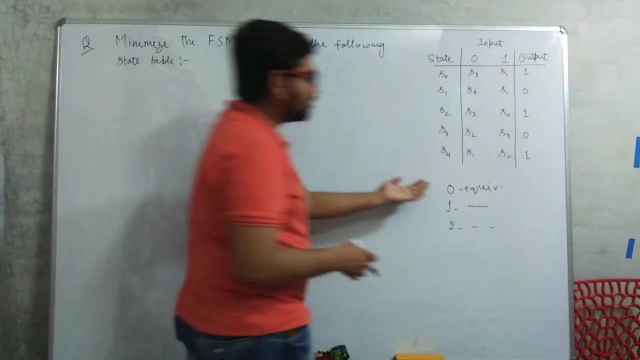 We define equivalence from start base. First of all, we will define 0 equivalence in its states. After defining 0 equivalence, 1 equivalence After 1, 2. We will keep going like this. Now, how far do we define this equivalence When we define 0 equivalence? 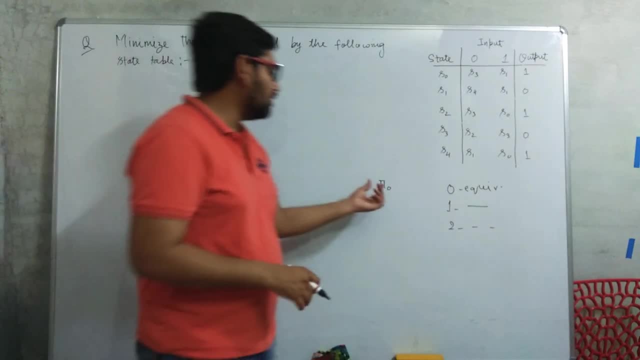 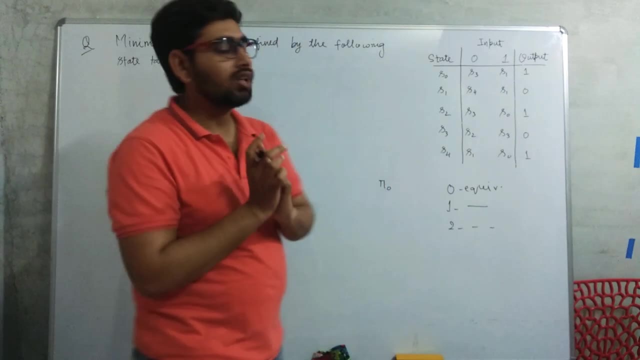 We will get a set of 0 equivalence. We will get a class of 0 equivalence, Which is denoted by pionauts. There will be such sets which will be 0 equivalent. There will be such states Which will be equivalent to each other. In the same way, we will get pi1. 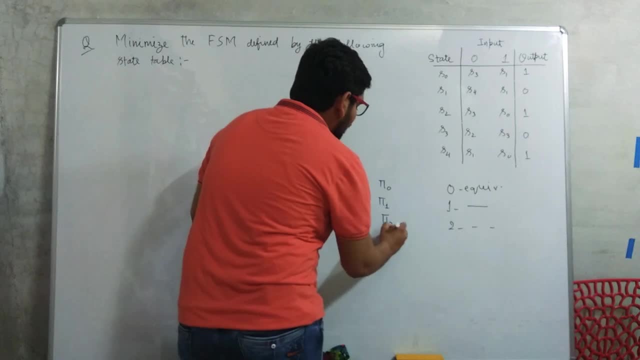 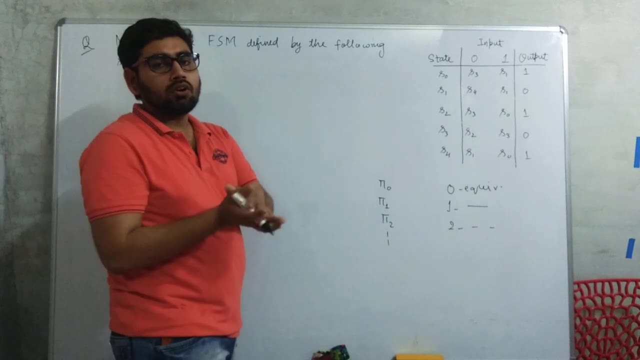 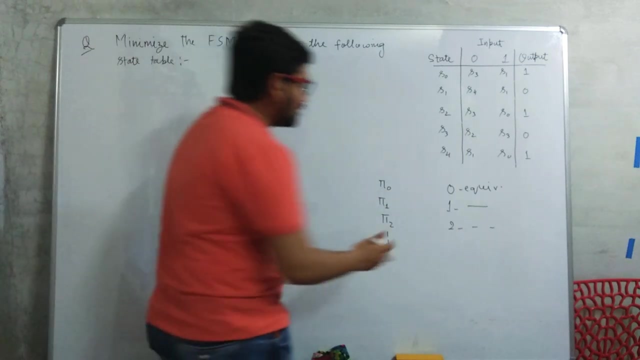 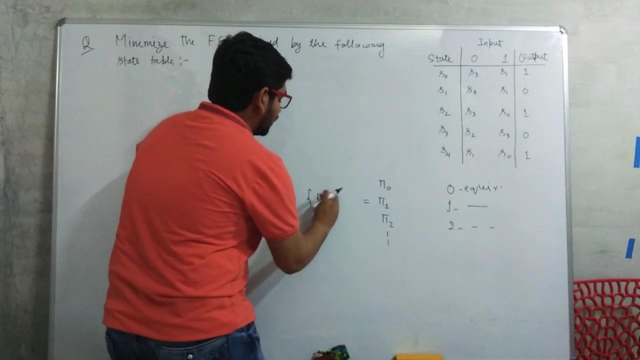 pi1, pi2. In this way we will get pi And we finish it there When we get 2 pi. Now states are there And equivalence is not being defined. In that case both will be equal. Consider pi1 In that S0 And S1, S0 and S1 came in one place. 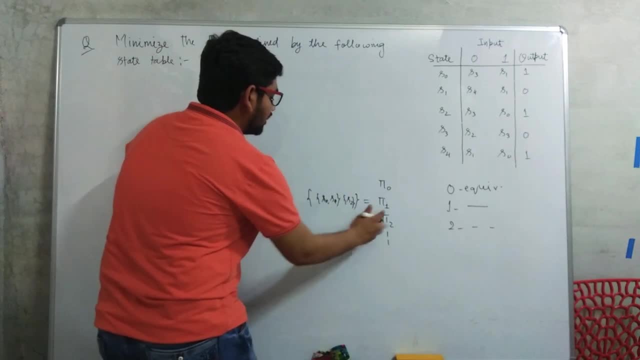 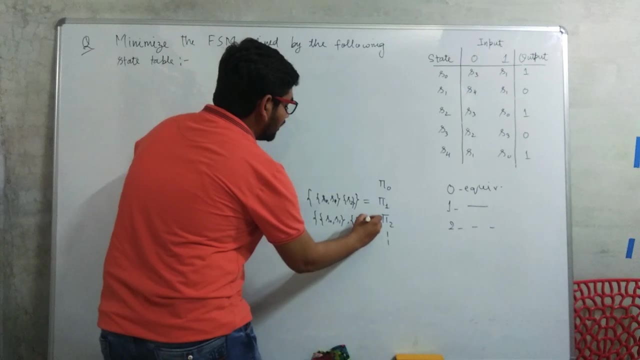 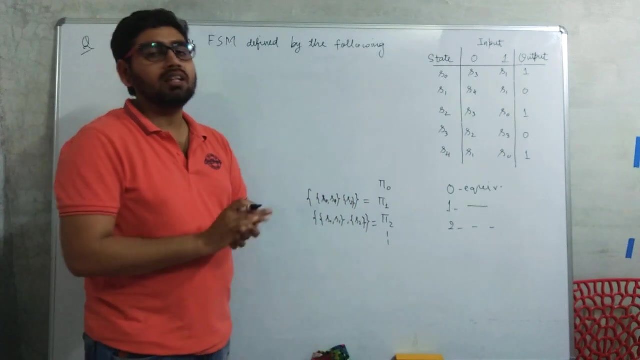 S2 came in one place In the same way. In the same way we got pi2, We got pi1 and pi2 We got the same. When they will start coming the same, Then this equivalence will be completed And these states We will get these states. We will call it k equivalent. 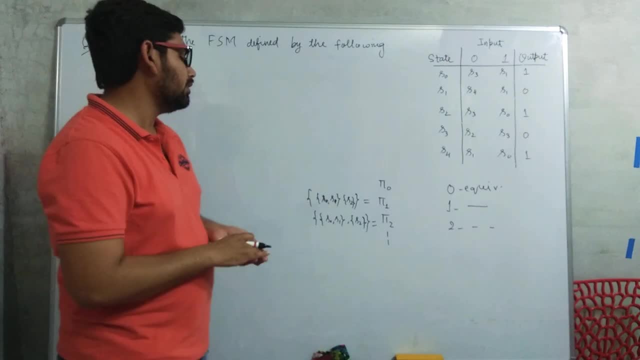 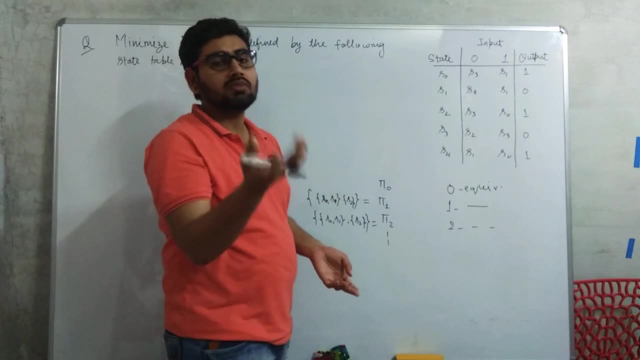 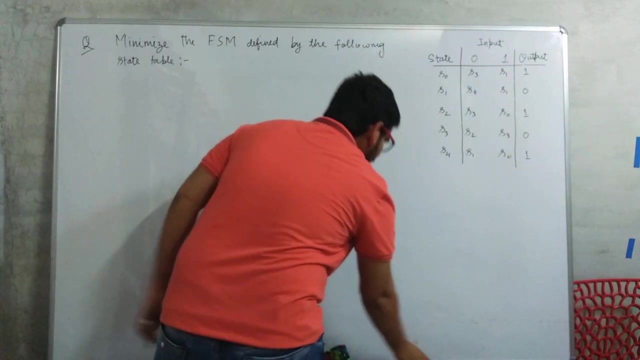 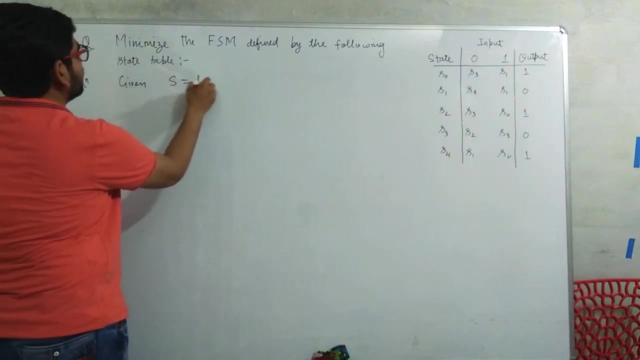 Means 2 equivalent or 1 equivalent. 2 equivalent will be 1 equivalent. We will call it 1 equivalent. So we will reduce these states In this table And we will define other machines. So Let's start with 0 equivalent. We have given Set of states, S. 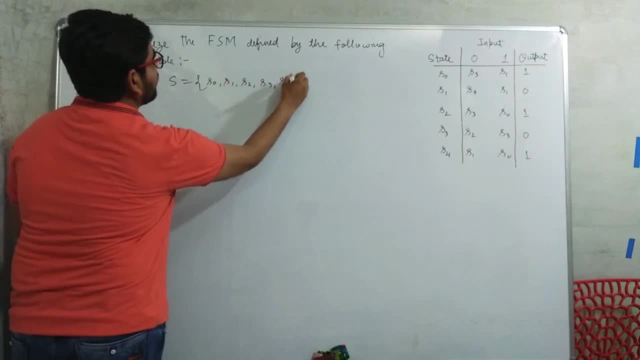 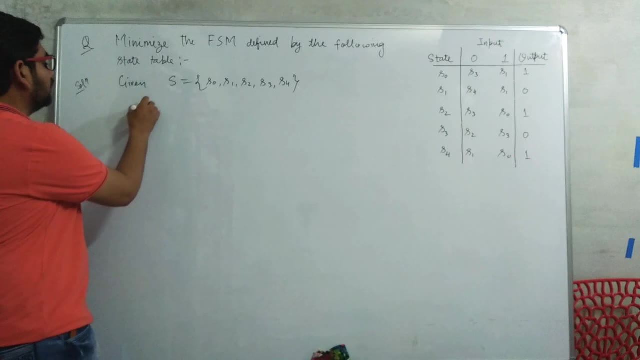 Which states are there: S0, S1, S2, S3 and S4. Now what we will do. First of all, we will try to find 0 equivalent states. We will write in pi0. In pi0 We will make sets of states Which will be 0 equivalent. 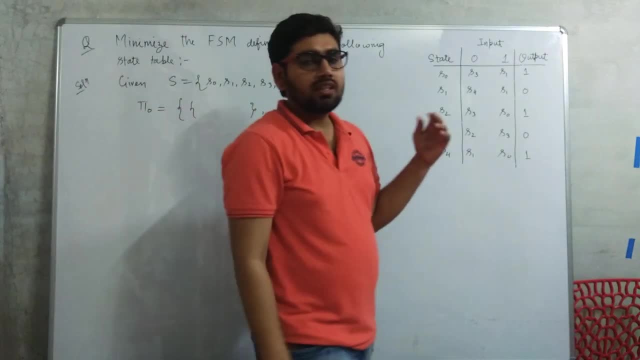 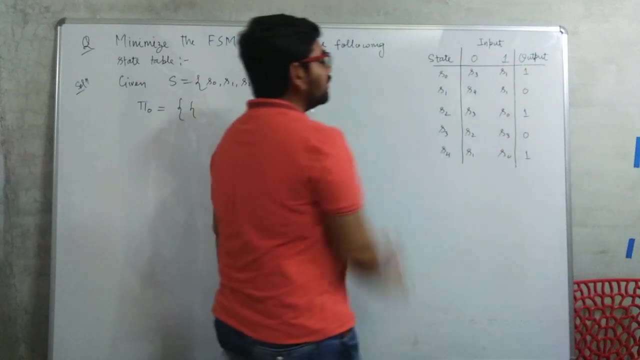 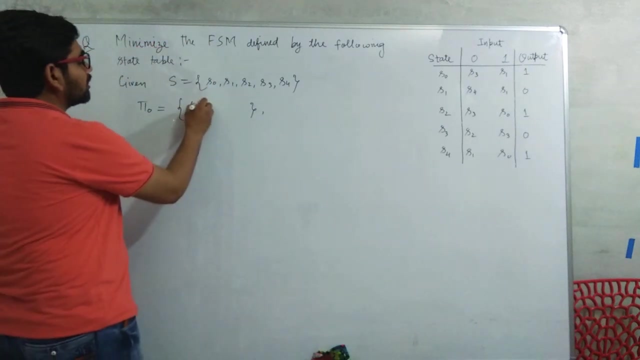 Their sets will be set. So to find 0 equivalent, We just have to see That the output is same. Output is: One output is corresponding to S0, One output is corresponding to S2 And one output is corresponding to S4. We can conclude from here That S0, S2 and S4 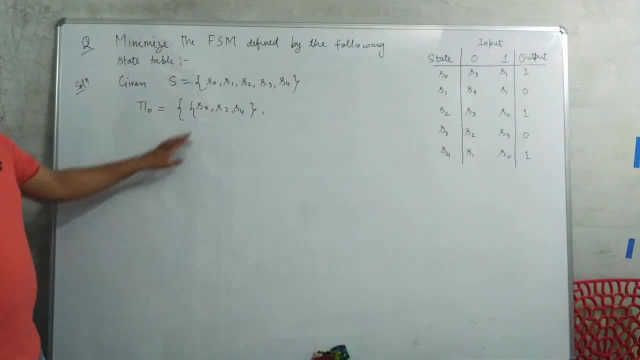 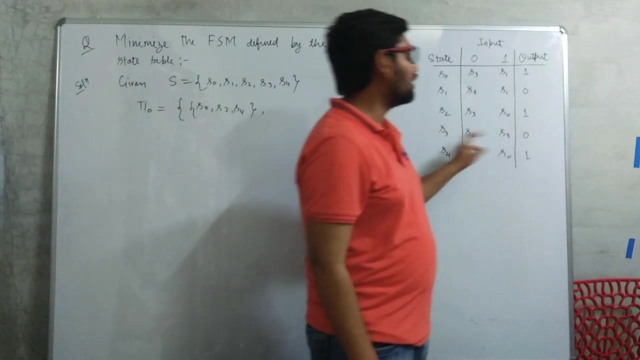 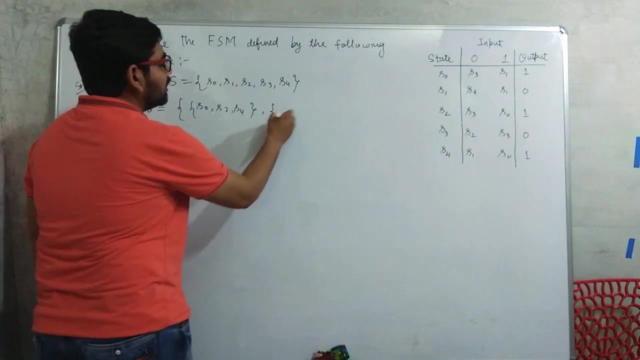 These are 0 equivalent states. These are 0 equivalent states By definition of 0 equivalent. We have to check the output. And the output of these states Is same. It means this is 0 equivalent. Similarly, 0 and 0 Output is same. So we can say: 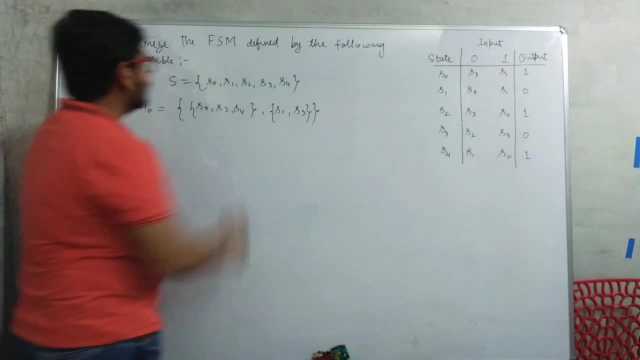 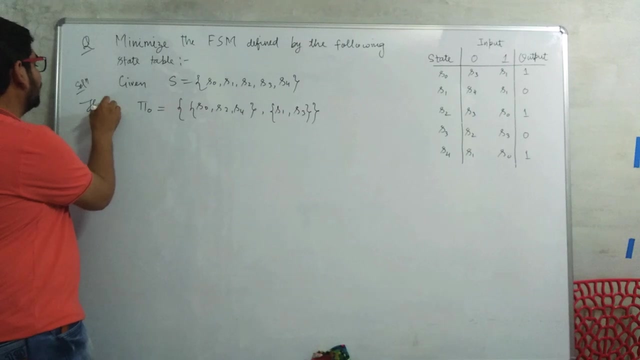 This will be 0 equivalent. So we have 2 sets of 0 equivalent And this is the collection Of those sets Which are 0 equivalent states. Then We will find pi1 And pi1. We will find such states Which are 1 equivalent. We have read the procedure. 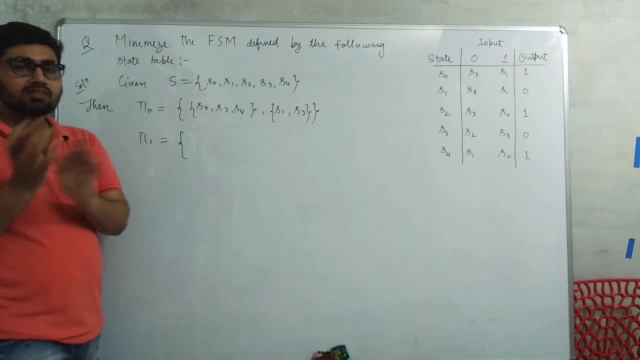 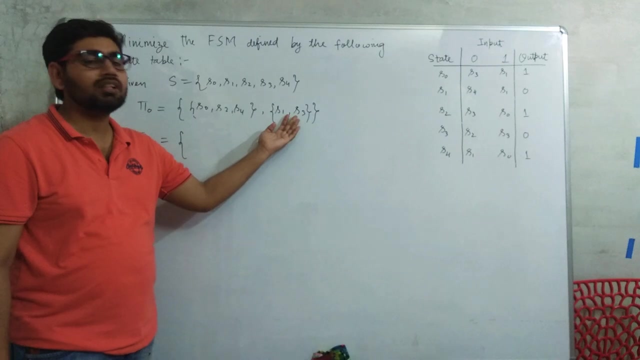 To find 1 equivalent. First of all, Their output should be same And the successive states Which we are getting, They should be 0 equivalent. So we will start from here First of all, In 1 equivalent. It will never happen. Here. the output is 0. How is their output? 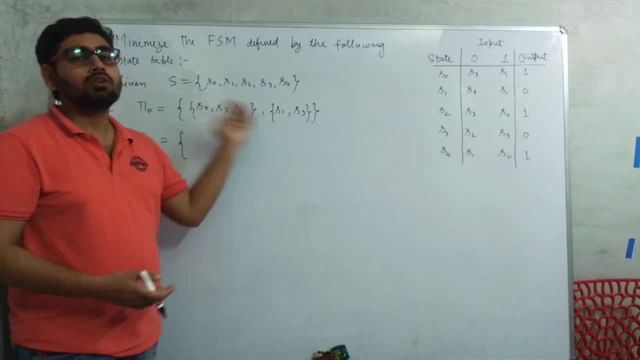 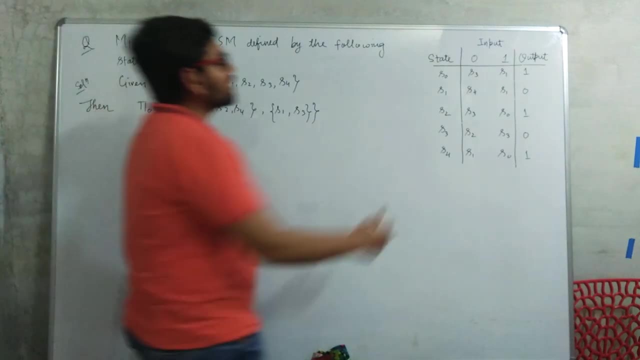 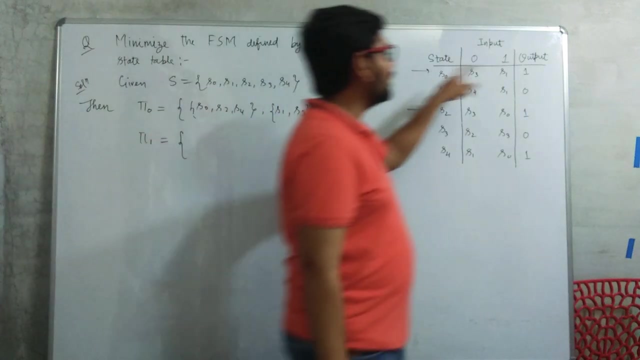 It is 1, Their output is different. So there will never be cross connection In cross. there will never be 1 equivalent. We will check S0 with S2 And S4 When we will check S0 with S2. One condition is being fulfilled, Their output is same. 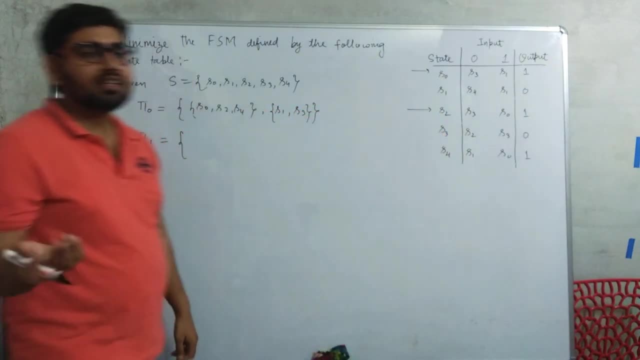 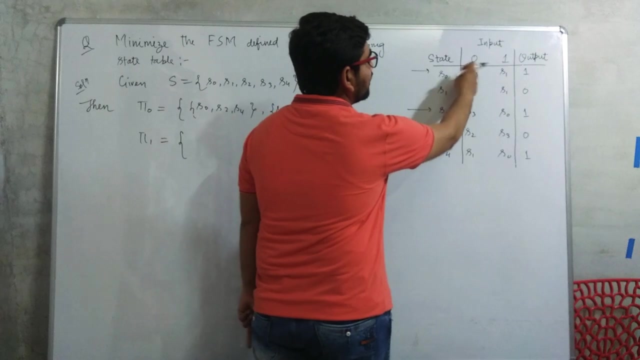 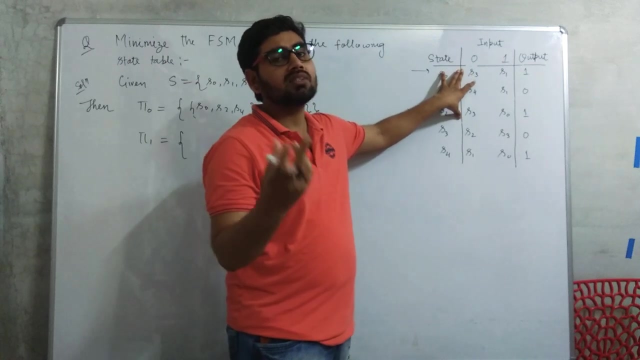 S0 has output 1. S2 has output 1. Now we have to see The successive states. When we give 0 input to S0, Then we get S3. When we give 0 input to S2, Then we get S3. Both the states are same. 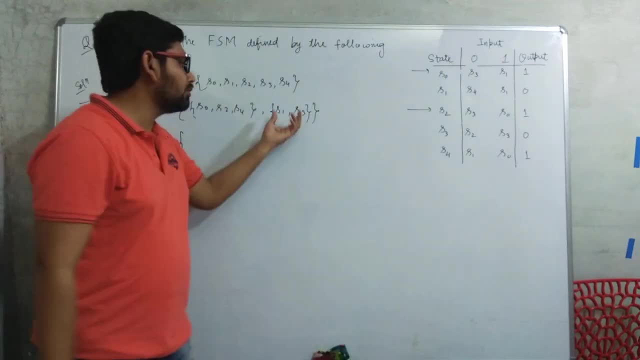 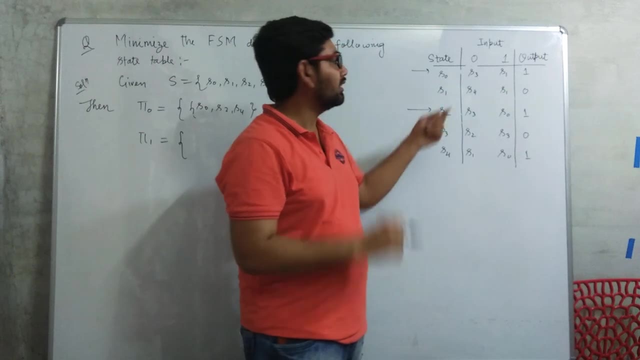 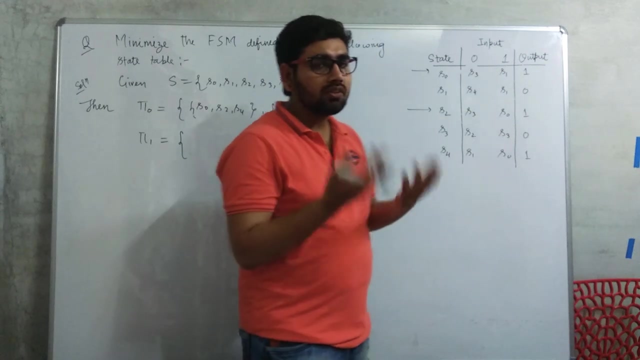 That means Both are 0 equivalent. They will be on the same side, In the same equivalence class. So this is 0 equivalent. Let's move forward. When we give 1 input to S0, Then S1 comes. When we give 1 input to S2, 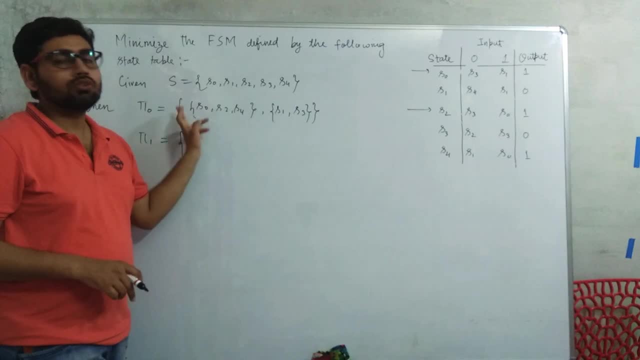 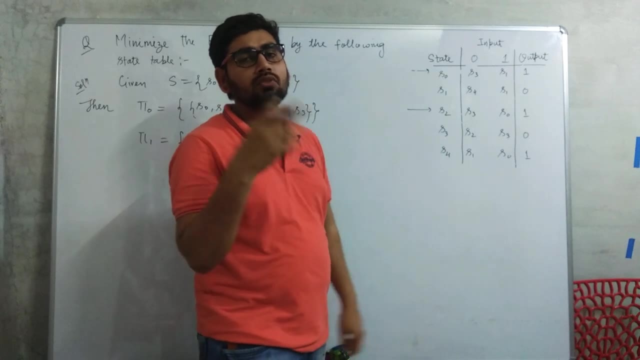 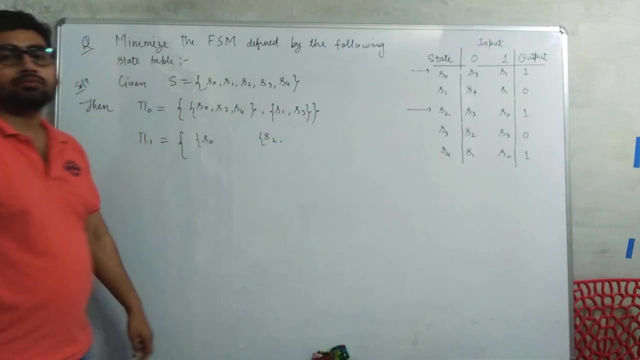 Then S1 and S0. They are not 0 equivalent. S1 and S0 are not 0 equivalent. It means Those who are checking S0 and S2, They are not 1 equivalent. That means S2 will not come in S0, S2 will come in another set. 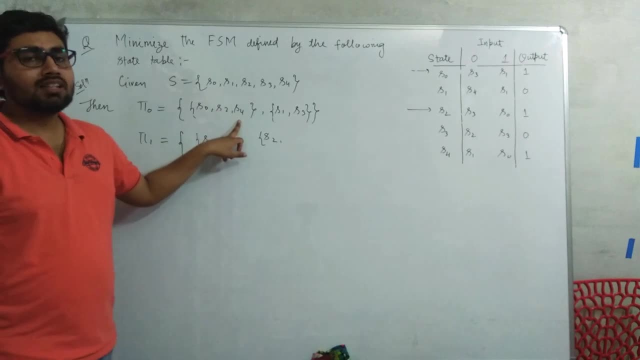 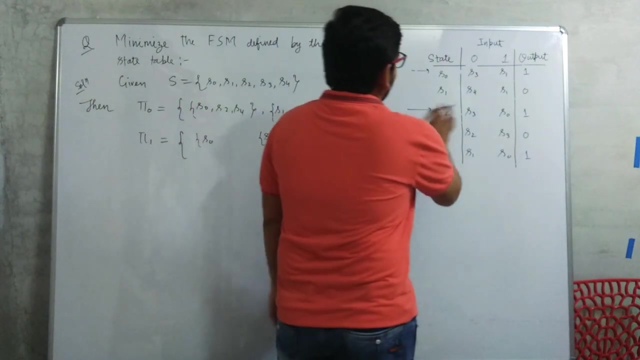 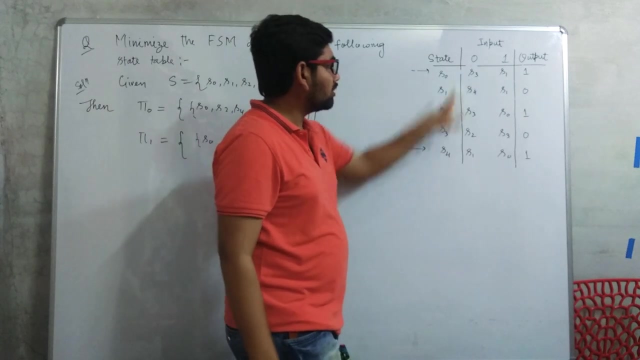 Now, S0 is not with S2. Let's check S0 with S4. Is S0 equivalent or not? Let's check S0 with S4. So Here, When we give 0 input to S0, Then we get S3, When we give 0 input to S4. 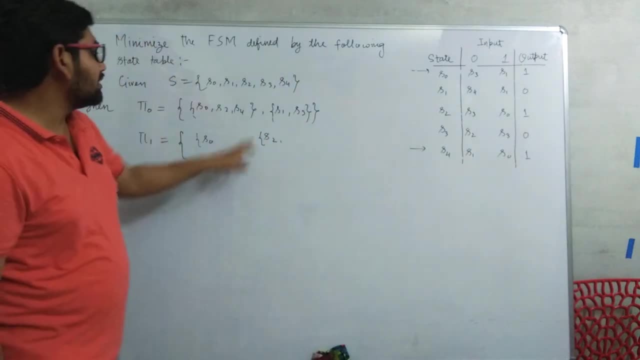 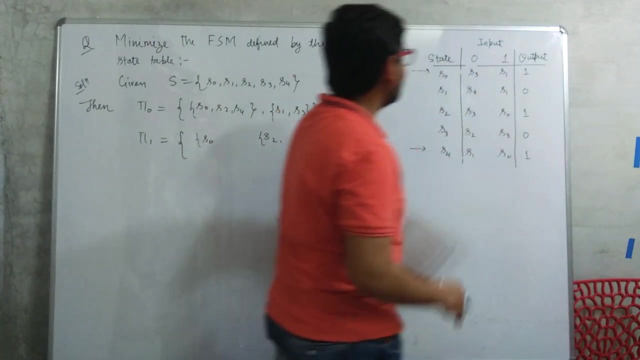 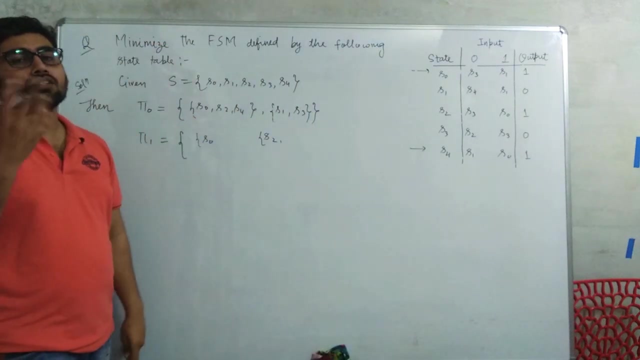 Then we get S1, S3 and S1. Both are 0 equivalent. Both are 0 equivalent. In the same way, When we give 1 input to S0, Then we get S1. When we give 1 input to S4, Then we get S0. 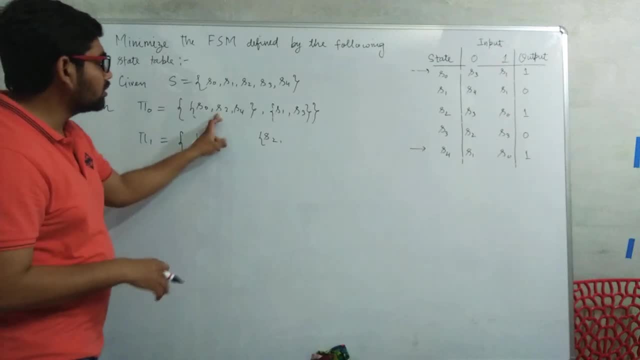 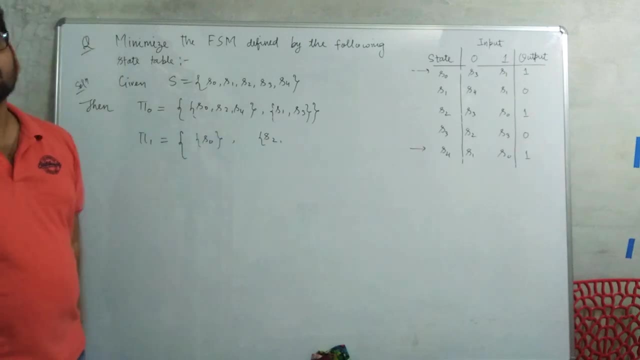 S1 and S0 are not 1 equivalent, It means S1 and S2 are not 1 equivalent. S1 and S4 are not 1 equivalent, Then S0 will come alone. Now let's see: Is S2 equivalent to S4, Then S0 will come. 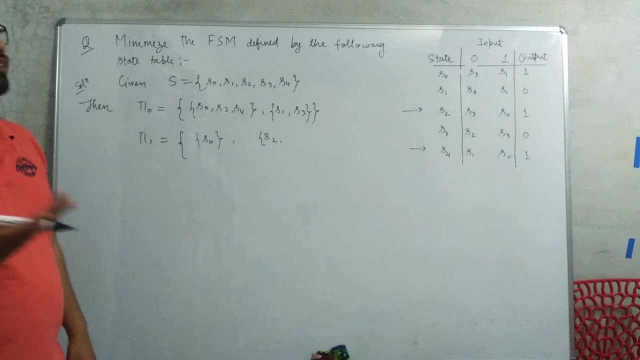 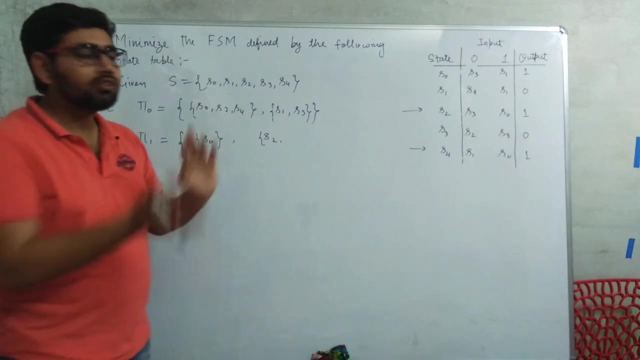 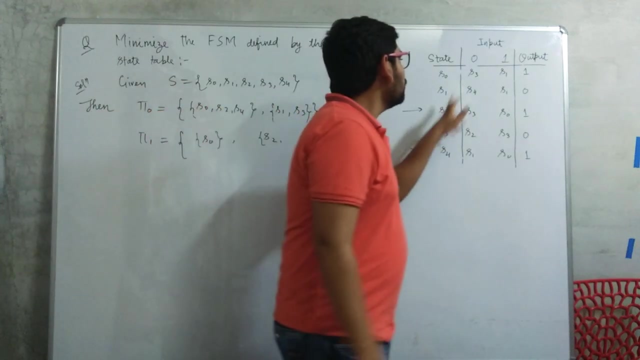 Let's check S2. Is S2 equivalent to S4? To check S2 equivalent to S4, Output is same. We just have to see What is the 0 equivalent. That means The previous equivalent Is in the same set: 0 input to S3, S4. 0 input to S1. 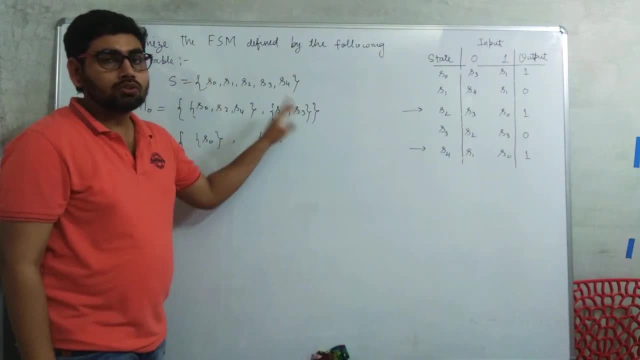 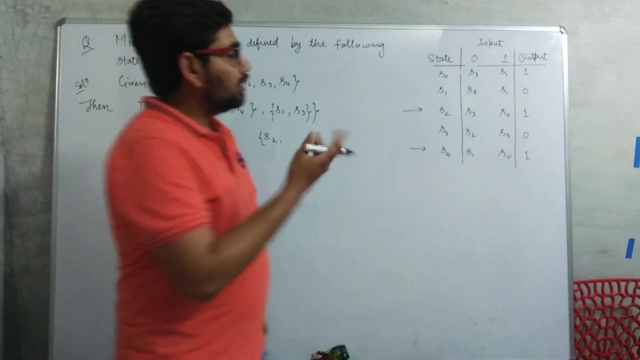 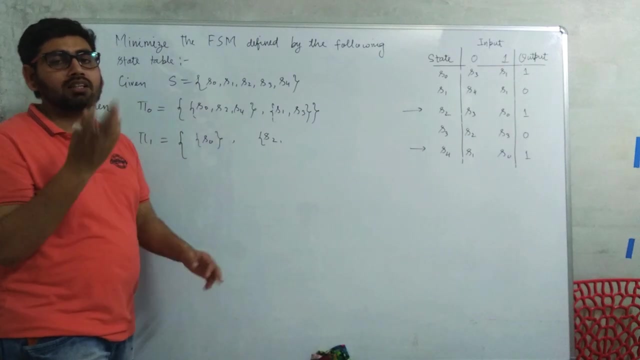 S3 and S1. Both are in the same class. That means both are 0 equivalent. S2 got 1 input to S0. S4 got 1 input to S0. From both, The output is S0 And S0 is same. That means both are in the same class. 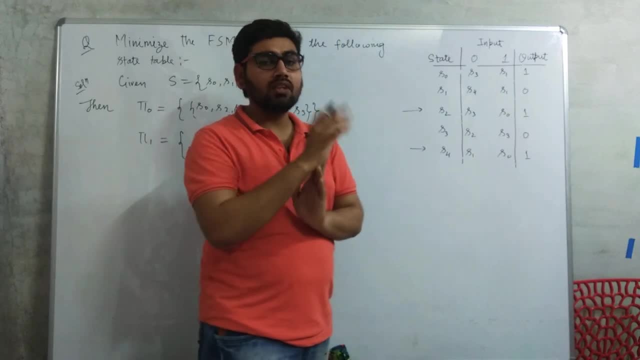 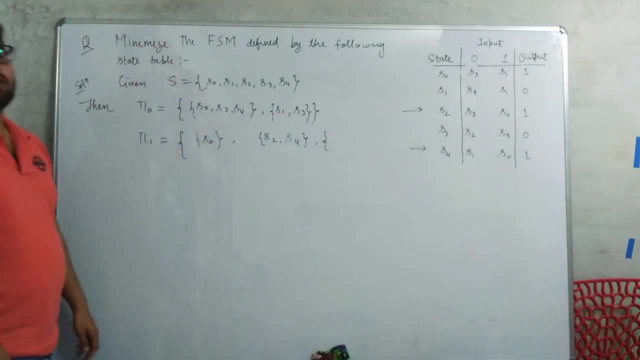 So the successive states of S2 Are 0 equivalent to each other. That means S2 is 1 equivalent to S4. S2 is 1 equivalent to S4. S2 is 1 equivalent to S4. S0 is not 1 equivalent to anyone. 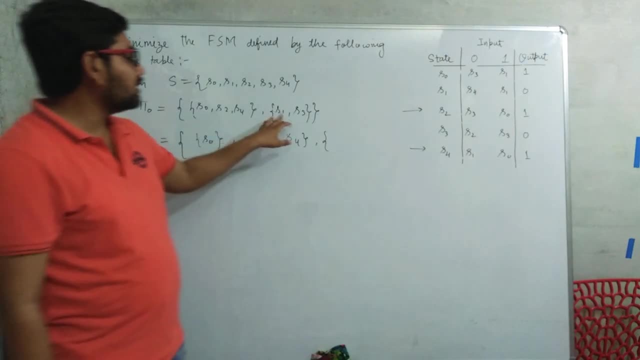 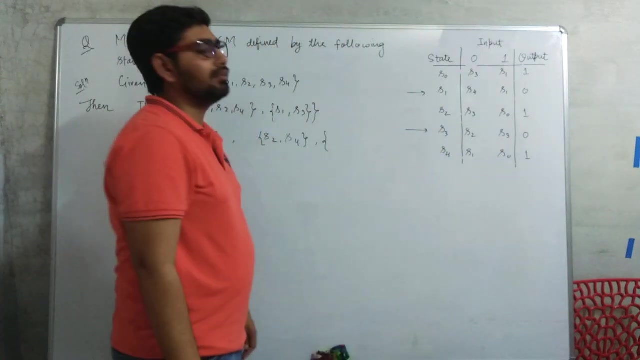 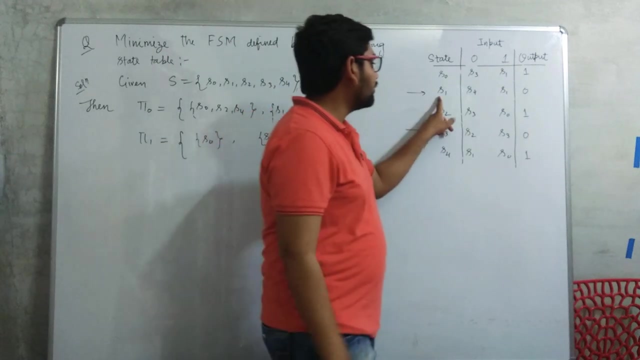 S2 is with S4. Now the remaining, We have to check S1 with S3, S1 and S3. We will check S1 and S3. Both have same output. We are checking them. Output is same. Let's see the successive states. Is it 0 equivalent? 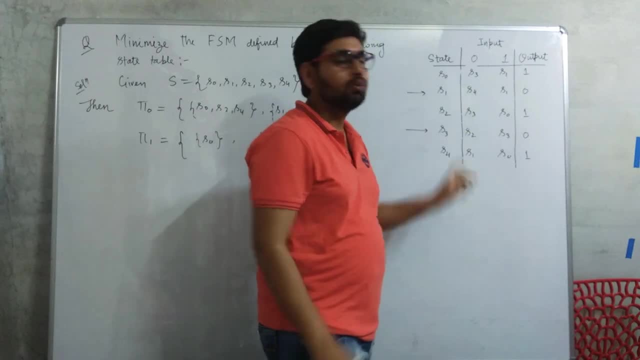 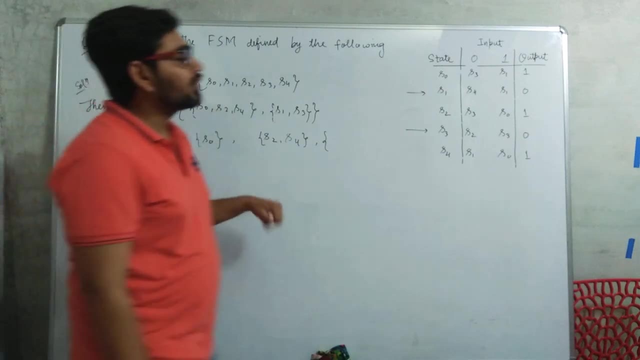 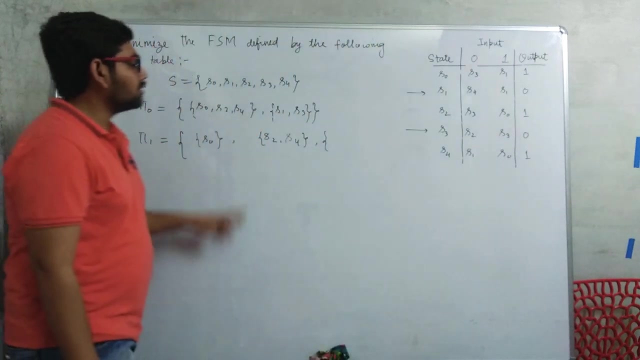 S3 got S2, S4 and S2. Is it 0 equivalent S4 and S2? Both are in the same class. That means both are 0 equivalent. S1 got 1 input. S1 got S3. S3 got S3. S1 and S3. 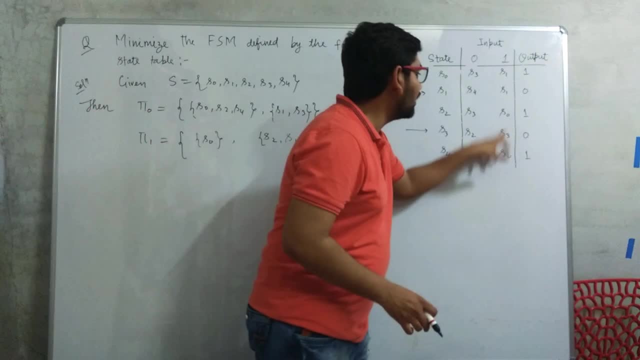 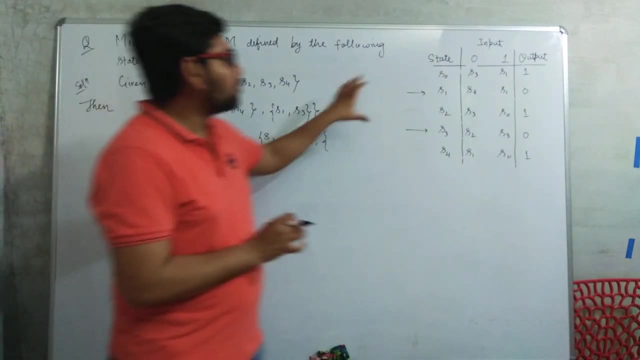 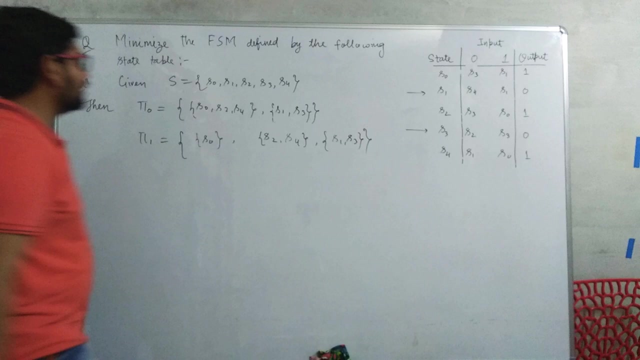 Both are in the same class: S1 and S3. Both are in the same class. That means both are 0 equivalent. 0 equivalent means successive states. Both are 1 equivalent. Both are in the same class: S1 and S3. The next We have 0 equivalent. 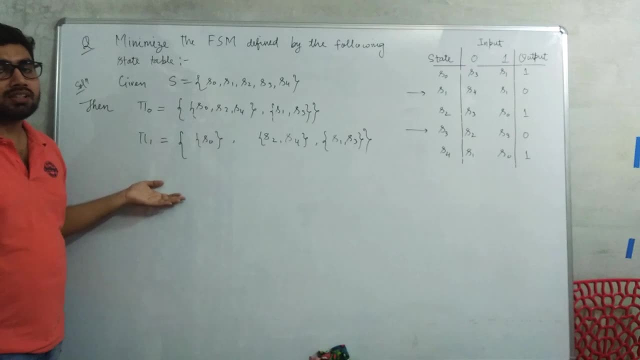 We have defined 1 equivalent. We will move like this: Finally, we will stop. This equivalence will come. We will define pi2. If pi2 is equal to pi1, We will stop here. We will find pi2. What we will do in pi2, We will see. 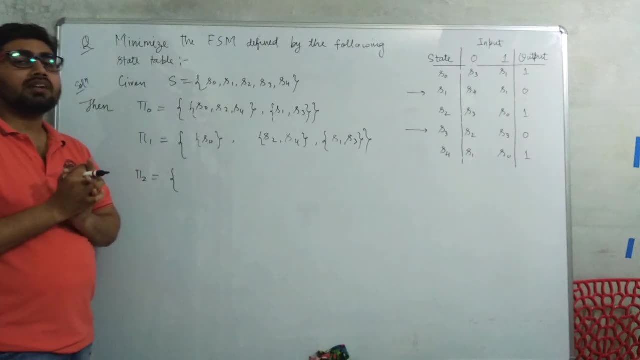 Now let's see what are the two equivalence states. To define two equivalence, we will take such equivalence classes In which two states are possible, In which state s0 is the only one. Here s0 is the only state. So this cannot be with two equivalents, Because it is not one equivalent. 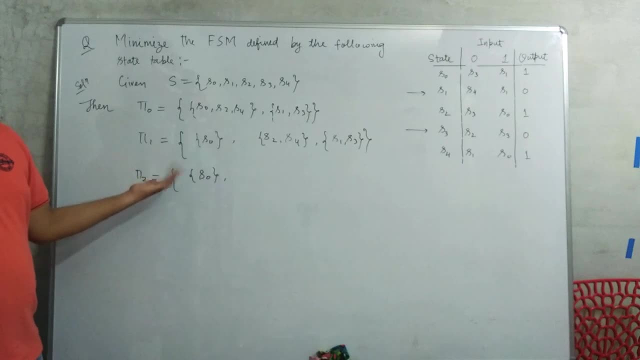 If it is not one equivalent, then it will not be two equivalent. S0 will be two equivalent with itself. So we have to check whether it is two equivalent or not. It is the same procedure to check two equivalents. s2 and s4 are in the same set. 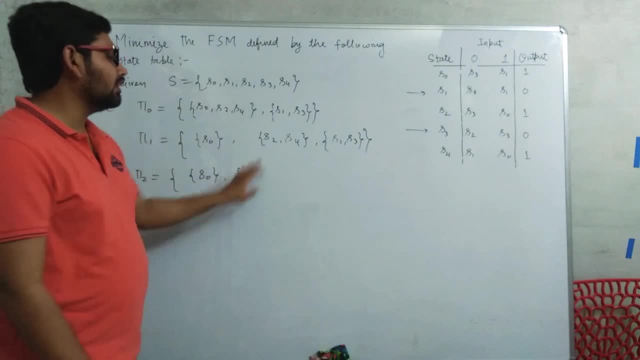 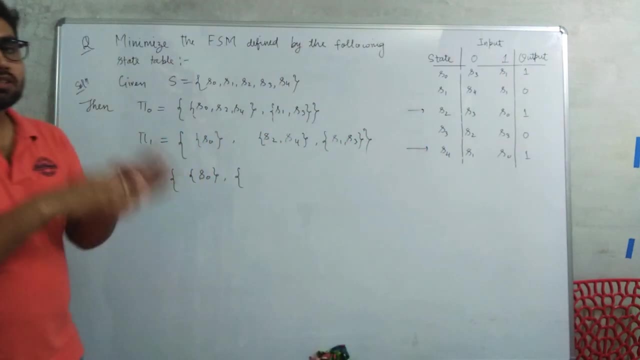 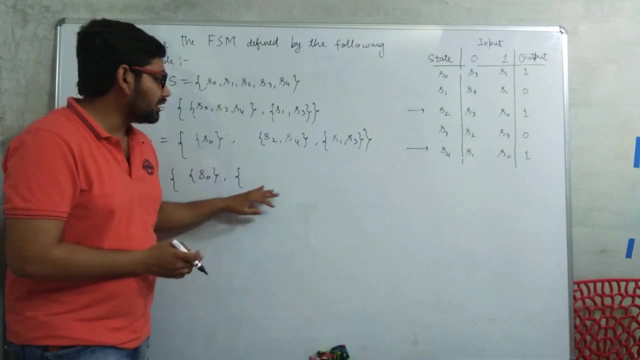 So we will check whether it is two equivalent or not. It is the same method to check two equivalents. So we have to check s2 and s4, The successive states of s2 and s4. The successive states will be given to them. Is it one equivalent? 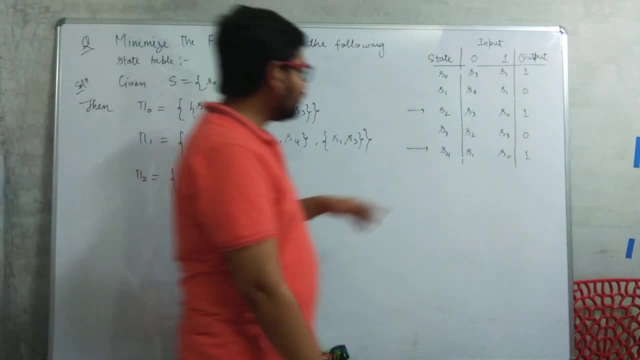 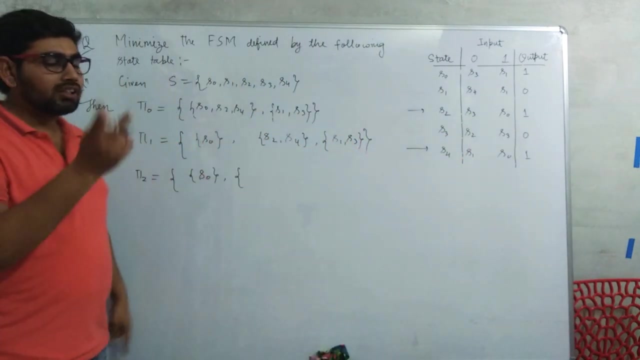 We used to check one in zero and two in one. If s2 is given to input zero, then s3. If s4 is given to input zero, then s1, s3 and s1 are in the same equivalence class. One equivalent s3 and s1. 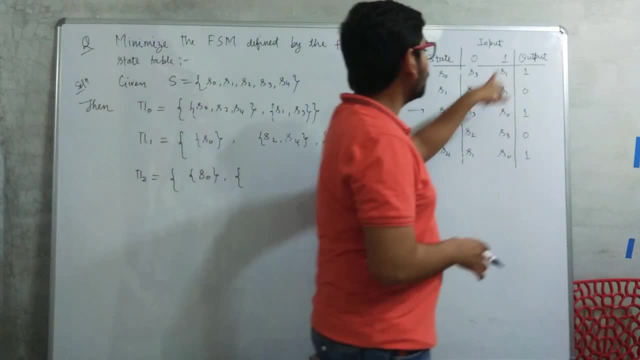 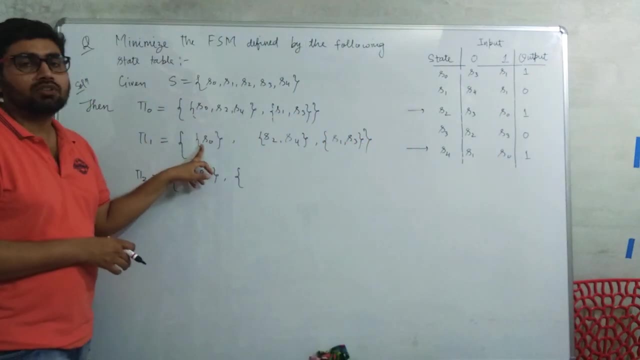 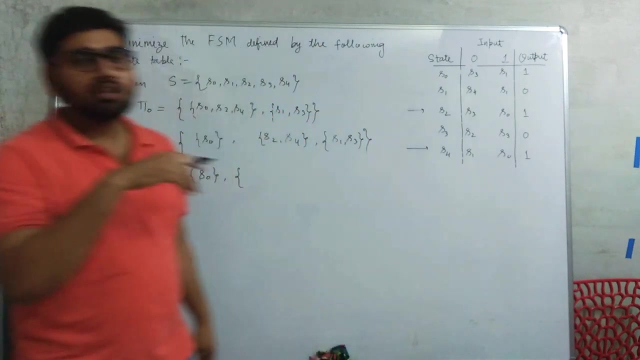 s3 and s1 are one equivalent. In the same way, s2 is given to input one, s0 is given to input one. Both are same. So both are happening. with s2 and s4, The successive states are in the same class. So we can conclude from here. 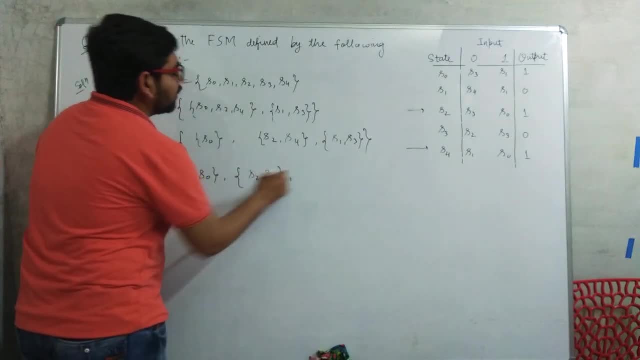 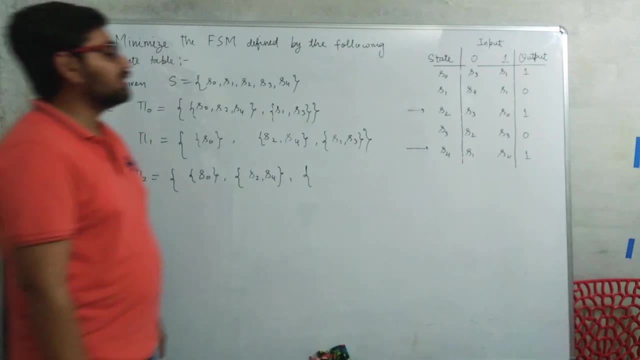 How are s2 and s4? They are two equivalent. Next, we will do for s1 and s3. We will check for s1 and s3. Both are in the same class So there is a possibility that they are two equivalent. To check two equivalents: s1 and s3. 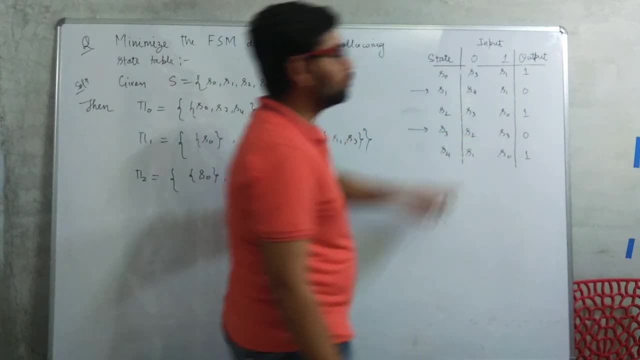 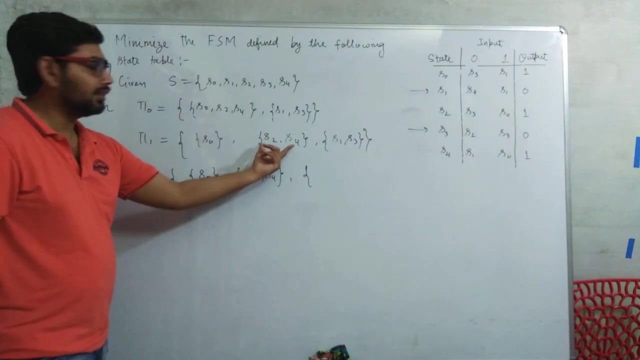 If s1 gives zero successive state, then s4. If s3 gives zero successive state, then s2. S4 and S2 are one equivalent in the same class. S1 is given as input. S1 and S3 is given as input. S3, S1 and S3 are one equivalent. Yes, 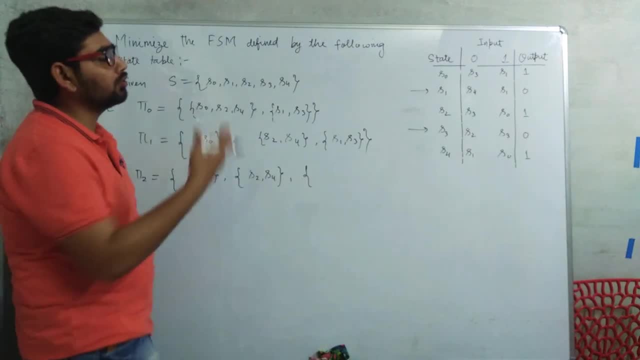 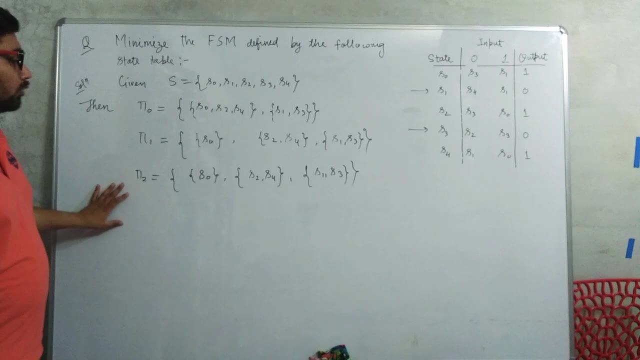 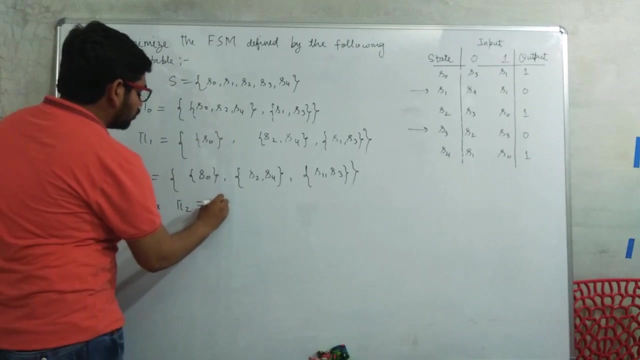 Both of them are one equivalent and two equivalent. So we have noticed that Pi1 and Pi2 are one equivalent of Pi1. We can conclude from here: Since Pi2 is equal to Pi1, The set of two equivalent states is equal to the set of one equivalent states. 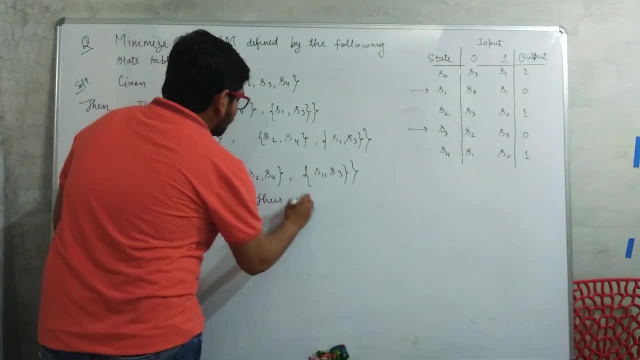 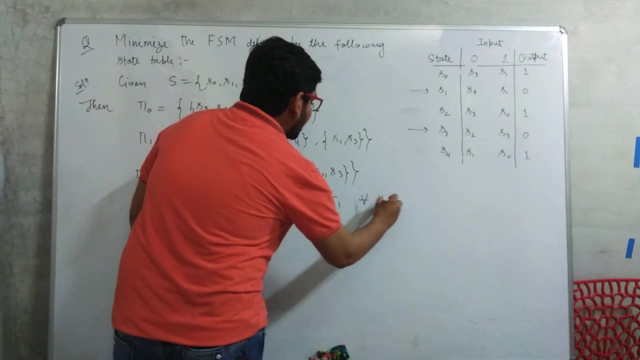 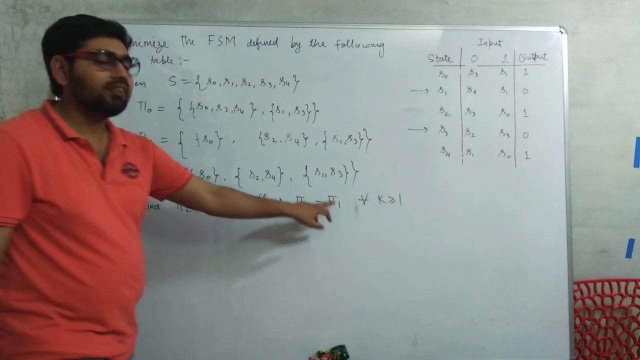 We can conclude from here. Thus: PiK will be equal to Pi1 For every K greater than or equal to 1. When K is greater than or equal to 1, Then whatever will come will be equal to Pi1. That means no equivalent is greater than or equal to 1. 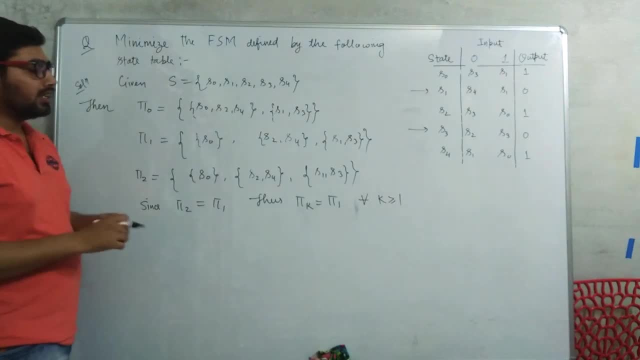 Then whatever will be equal to Pi1 will be equal to Pi2, So we can conclude from here That we have got the equivalent states. The final equivalent state of S0 is only of S2 and S4 And S1 is of S3. Now we have to minimize the finite state machine. 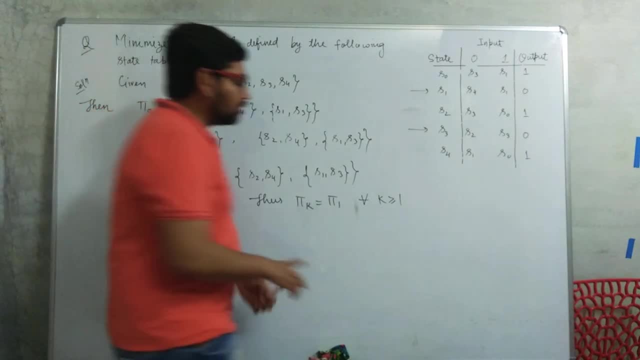 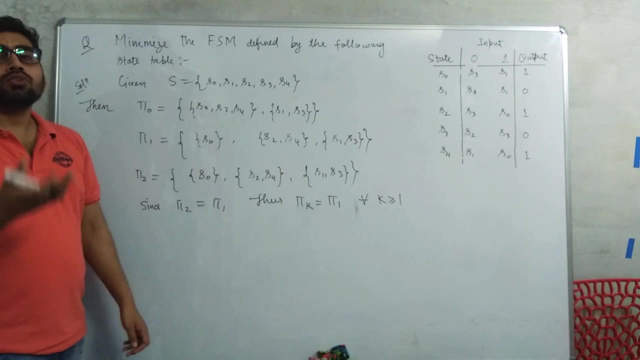 Because we have to minimize the finite state machine. So we have to reduce the states. We have to reduce the states. Finally we have the equivalent states. We will remove the states which are equivalent to each other And we will leave the other states, For example. Finally we have the result. 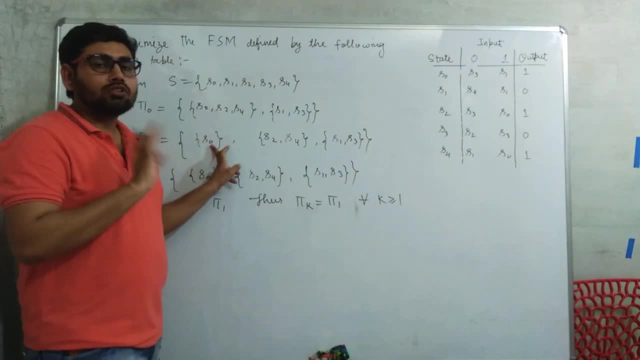 Take Pi1 and Pi2. S0 is not with anyone, So we will retain S0. We will keep it. S2 and S4 are equivalent, So we will reduce S4. We will write S2 instead of S4. Okay, S1 is equivalent to S3. 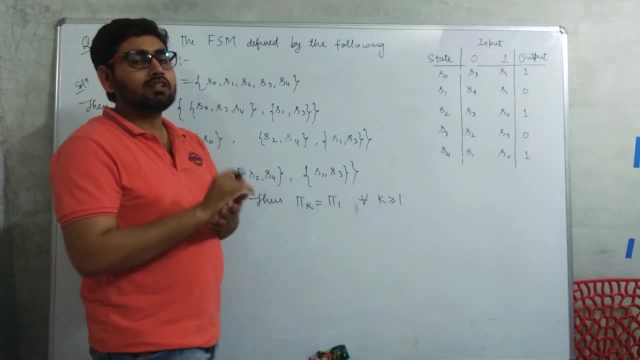 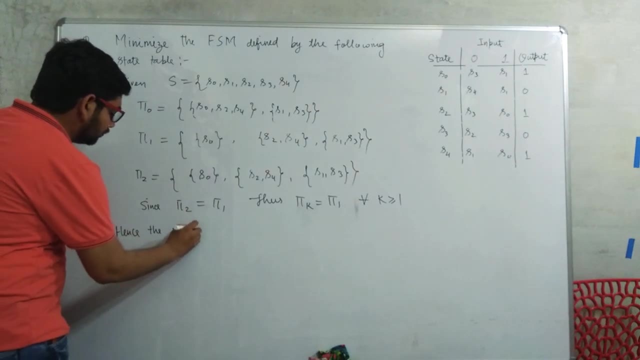 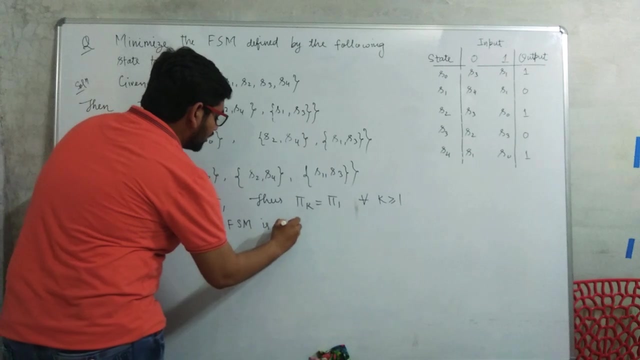 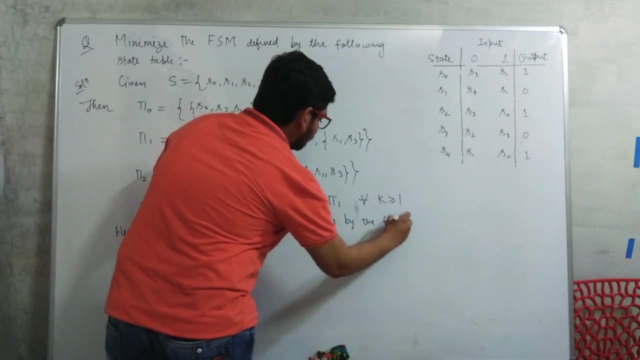 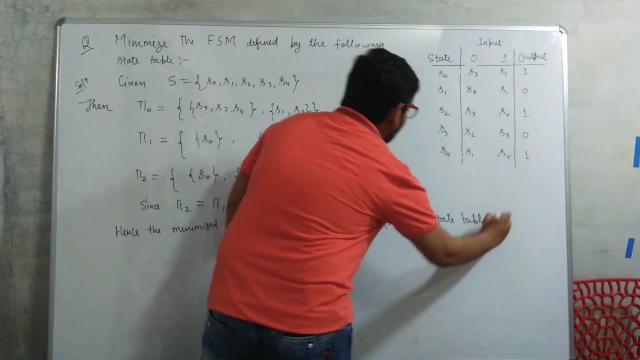 So we will remove S3 and S1 Remove any one. Rest of the states will be saved. Hence The minimized finite state machine is represented by the following state table: The minimized finite state machine is represented by this state table. The minimized finite state machine is nested at P3. 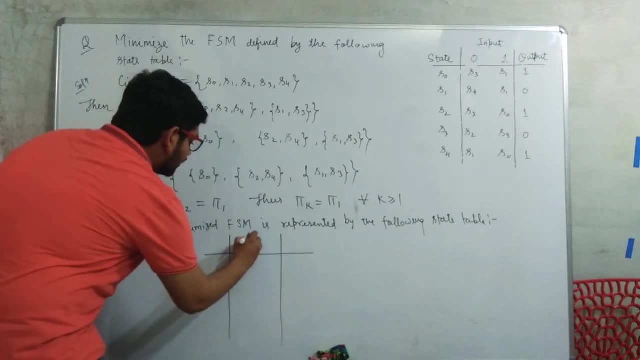 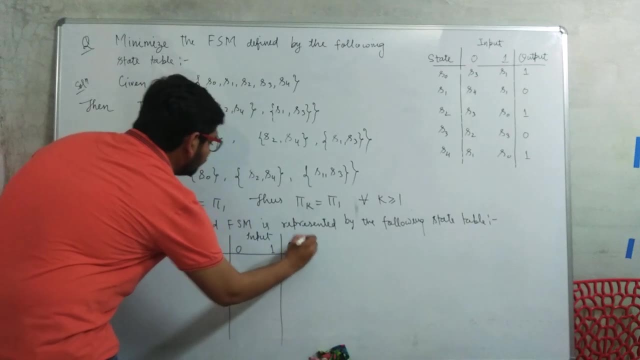 The minimized finite state machine is represented by this state table. The minimized finite state machine is set to the setting of independent states And the rest of the states will go back to existing state. For example, P3, P2, P3, P2, P3, P3, P3. 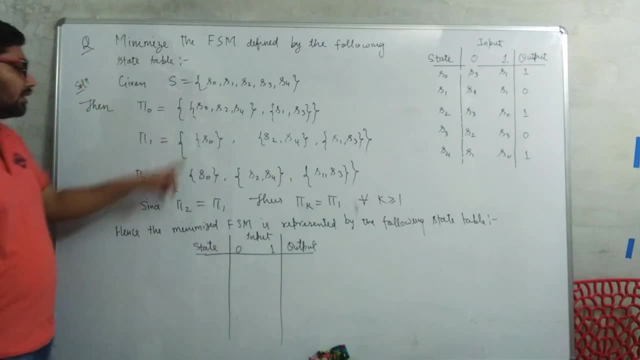 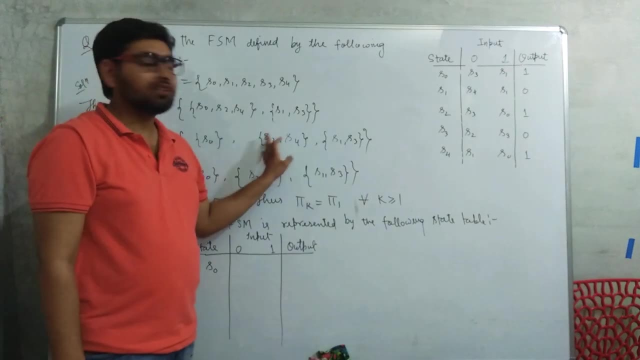 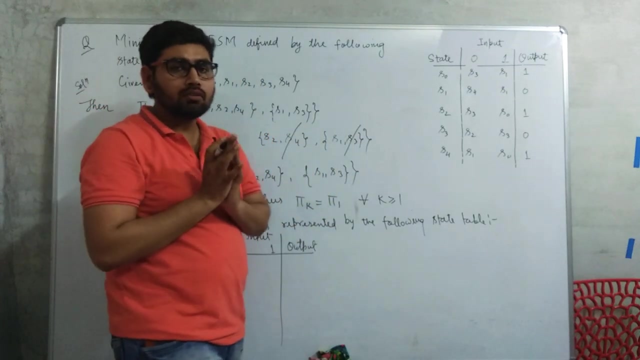